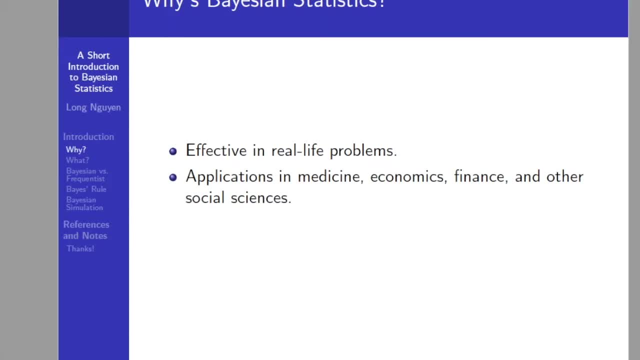 new data comes in. It has a lot of application in quantitative finance, economics, medicine and other social sciences. In finance, quantitative traders make heavy use of Bayesian inference and application of Bayesian statistics with time-series analysis to predict future values. What is Bayesian statistics? As stated above, Bayesian statistics is one of many approaches. 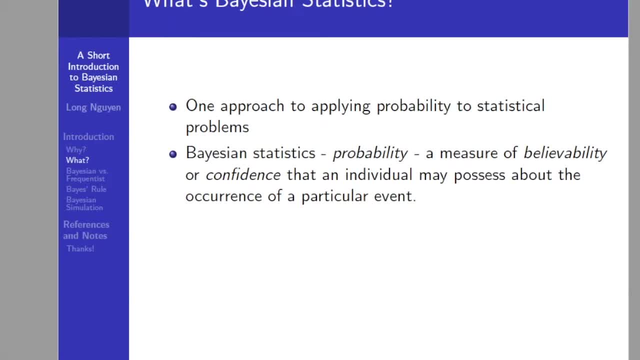 to probability. Bayesian statistics consider probability as a measure of believability or confidence that an individual may possess about the occurrence of a particular event. We may have a prior belief about an event, but our beliefs are likely to change when new evidence is brought up. Bayesian statistics. 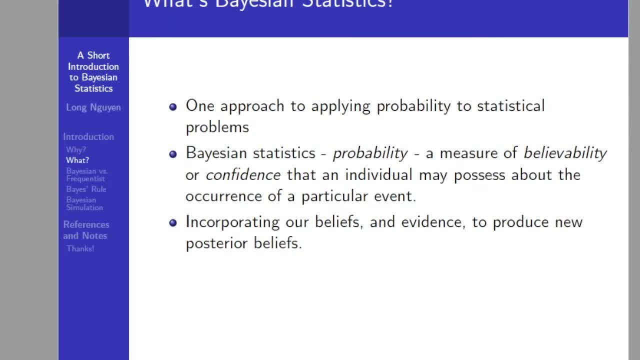 gives us a solid mathematical means of incorporating our beliefs and evidence to produce new material beliefs, which assumes that probabilities are the frequency, not the frequency of a particular random event occurring in the long run of repeated trials. For example, as we roll a fair, unweighted six-side die repeatedly, we would see that each number on 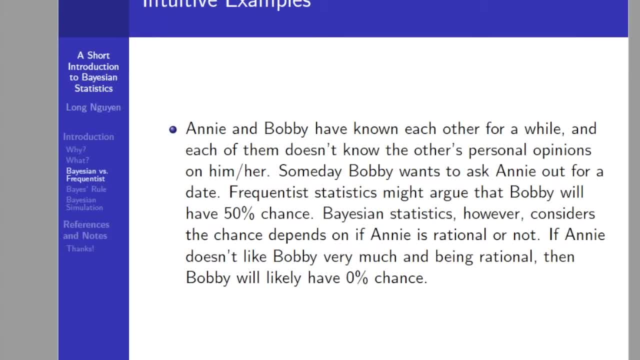 the die tends to come out one, six at a time. Let's think about an intuitive example. Annie and Bobby have known each other for a while and each of them doesn't know the other personal opinions on him or her. Some day Bobby wants to add Annie out for a date. Frequent statistics might argue that Bobby will have. 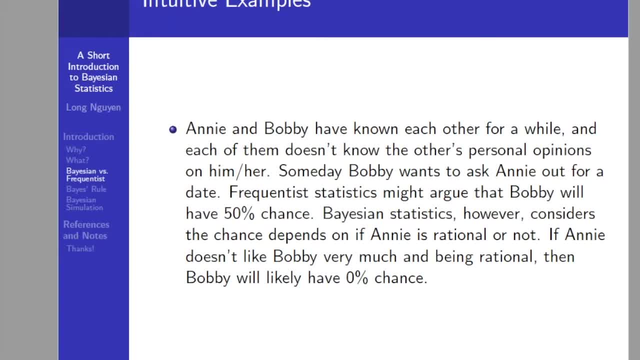 50% chance of winning the date, But on the other hand, Bayesian statistics, however, consider the chance depends on if Annie is rational or not. If Annie doesn't like Bobby very much and being rational here, then Bobby will likely have 0% chance. Let's take a closer look at the difference between. 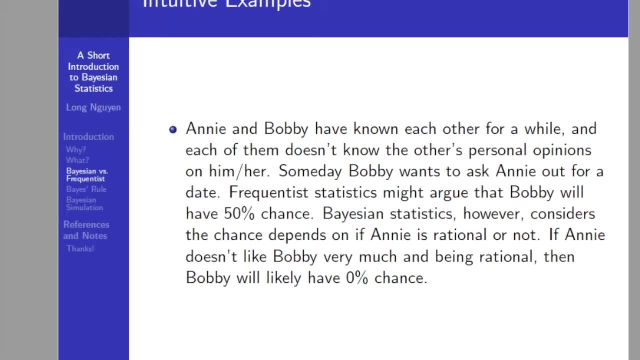 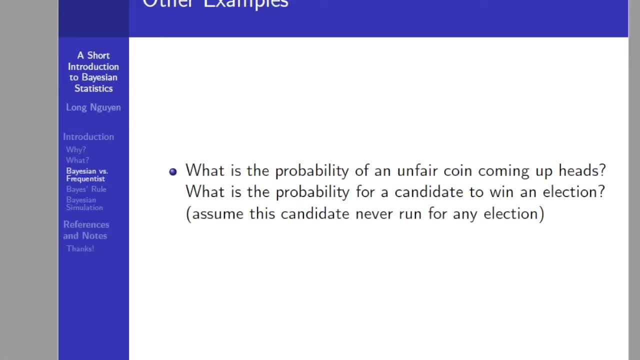 Frequencies statistics and Bayesian statistics by the two examples. So what is the probability of an unfair coin coming up ahead and what is the probability for a candidate to win an election? and assume this candidate never runs for any election? About the unfair coin flip: 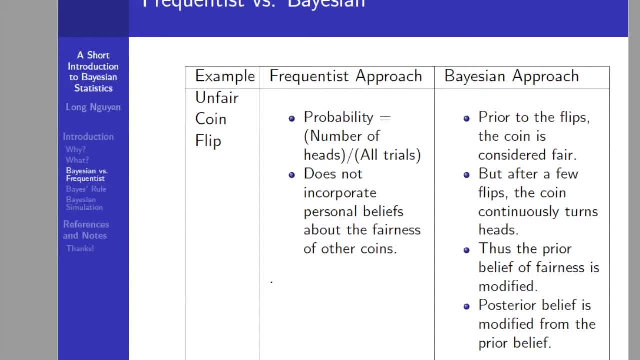 on Frequencies approach, the probability of seeing a head when the unfair coin is flipped is around long-run relative frequency of seeing a head when repeated flips of the coin are carried out. As we carry out more coin flips, the number of heads obtained as a proportion of the total. 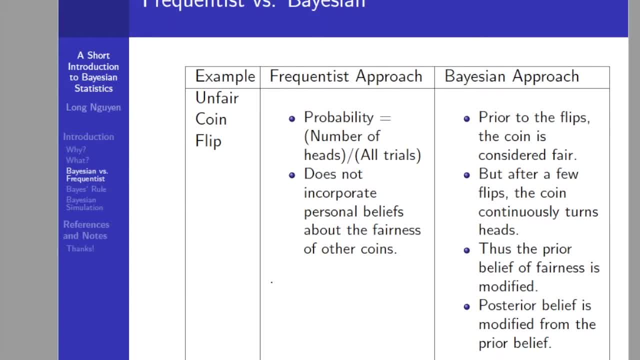 flips tends to be the true or physical probability of the coin coming up as heads. In particular, the individual running the experiment does not incorporate his or her own beliefs about the fairness of other coins. On the other hand, on the version of ProSci, prior to any flip of the coin, a person may 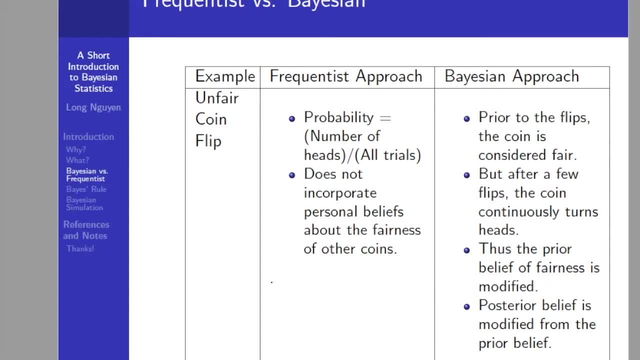 believe that the coin is fair. After a few flips, the coin continually comes up heads. Thus the prior belief about fairness of the coin is modified to account for the fact that, for instance, 3 heads have come up in a row and thus the coin may not be fair After 500 flips with 400 heads, the person 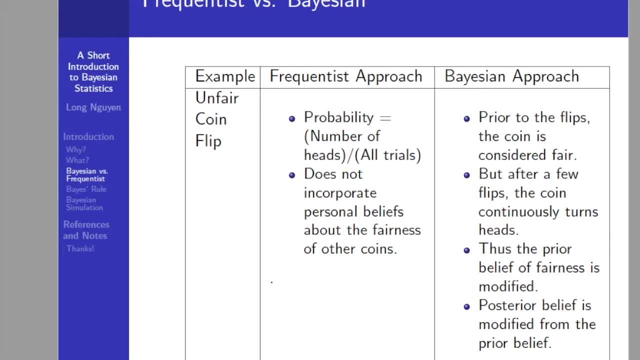 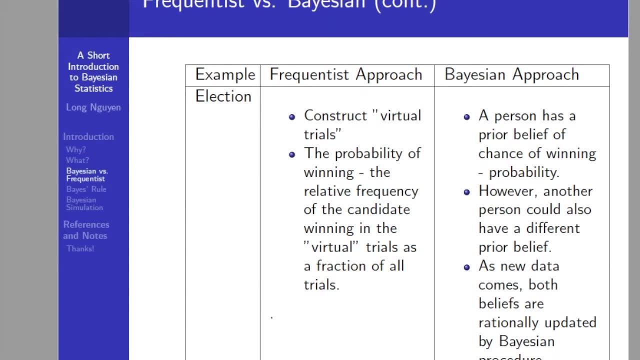 believes that the coin is very unlikely to be fair. The posterior believes it is heavily modified from the prior belief of an unfair coin. About the election example: on the frequentist approach side the candidate only ever stands once for his particular election, so we cannot perform repeated trials here In a frequentist. 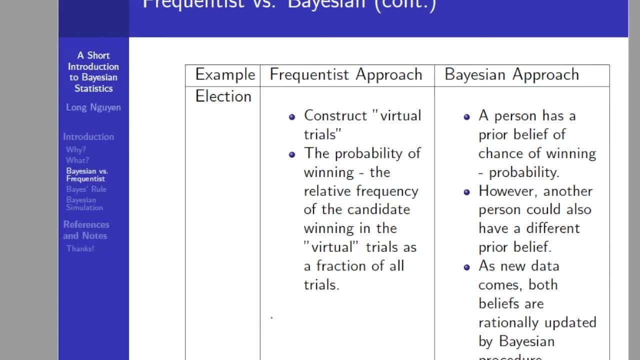 point of view, we construct virtual trials of the election process. The probability of the candidate winning is defined as the relative frequency of the candidate winning in the virtual trials as a fraction of all trials. On the other hand, on the Bayesian approach side, 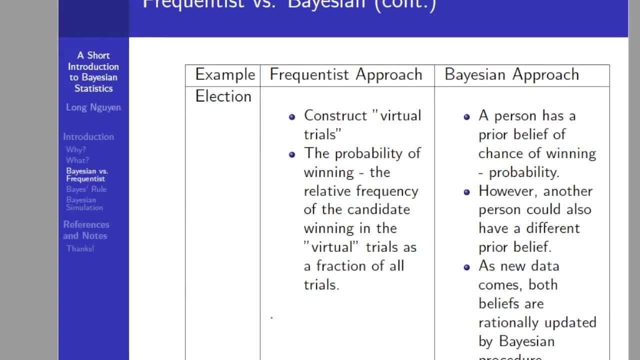 a person has a prior belief of a candidate's chance of winning an election and that person's confidence can be quantified as a probability. However, another person could also have a different prior belief about the same candidate's chances. As new data comes, both beliefs are rationally. 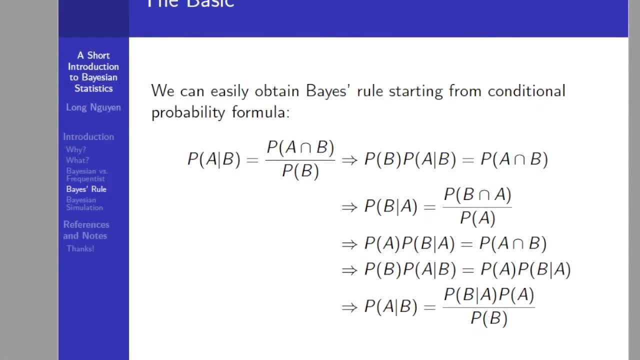 updated by the Bayesian procedure. As some of you might have heard or known about the famous Bay rule, actually the Bayesian rule can be obtained from conditional probability formula. Here the process of obtaining the Bayesian rule is very easy. The whole process would take about 5 lines. 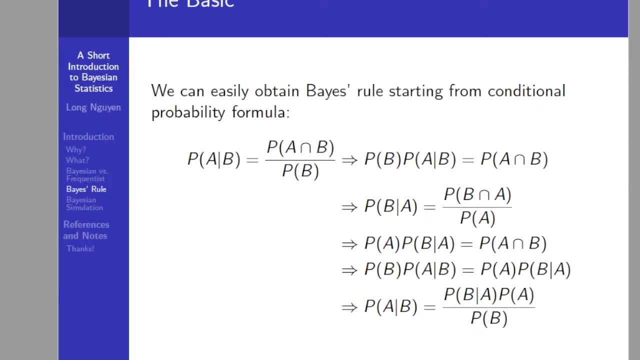 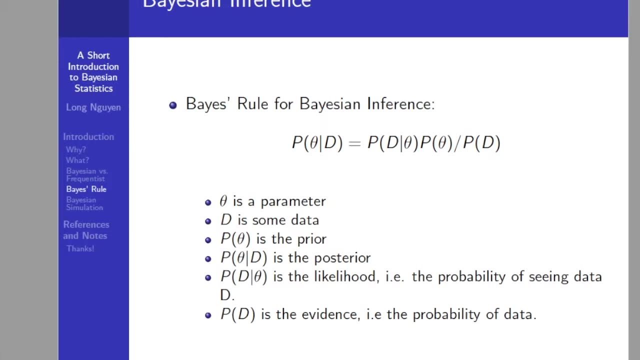 But actually remember here the probability of A intersect B equals the probability of B intersect A. That's the only thing I want to remind you. Now we can use Bayes' rule To demonstrate a concrete numerical example of Bayesian statistics. there are two important 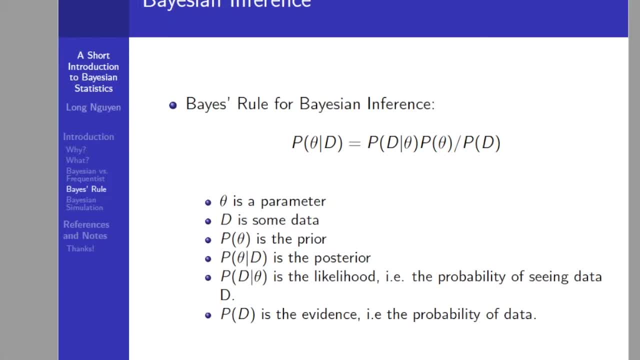 concepts, parameters and models. A parameter could be the weighting of an unfair coin which is labeled as theta. Thus, theta equals p of h. would describe the probability distribution of our beliefs that the coin will come up at h when flipped. The model is the actual. 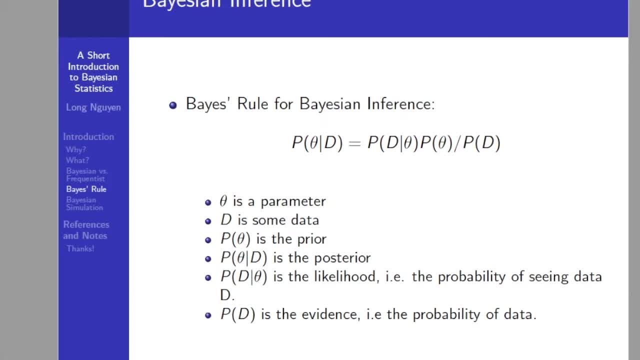 means of decoding this flip mathematically. For example, the coin flip can be modeled as a Bernoulli child. It's also very important to know about Bayes' rule for Bayesian inference. Bayesian inference can be written as: p of theta given d equals p of d given theta times p of theta over p. 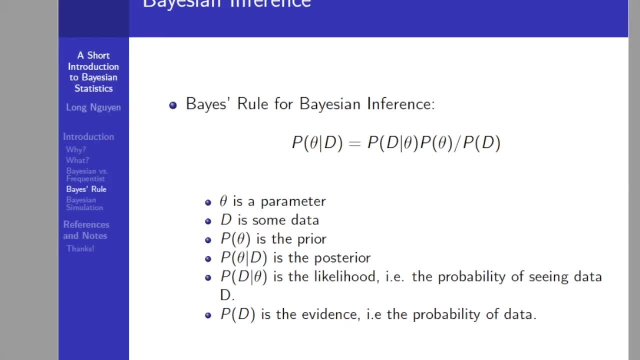 d. p of theta is the prior. This is the strength of our belief that the coin will come up at h, without considering the evidence d, Our prior view on the probability of how fair the coin is. p of theta given. d is the posterior. This is the strength of our belief of theta. 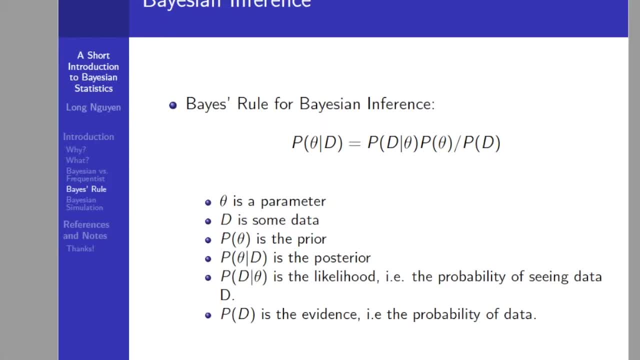 once the evidence d has been taken into account. For example, after seeing four heads out of eight flips say: this is our belief that the coin will come up at h when flipped. This is the strength of our belief that the coin will come up at h after seeing four heads out. 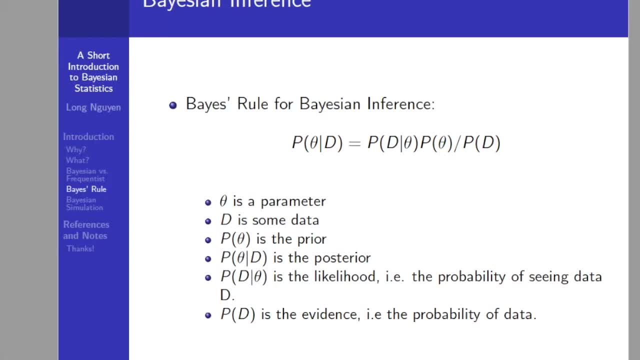 of eight flips. This is the strength of our belief that the coin will come up at h after seeing four heads out of h. This is our updated view on the fairness of the coin. p of d: given theta is the likelihood, This is the probability of seeing the data. 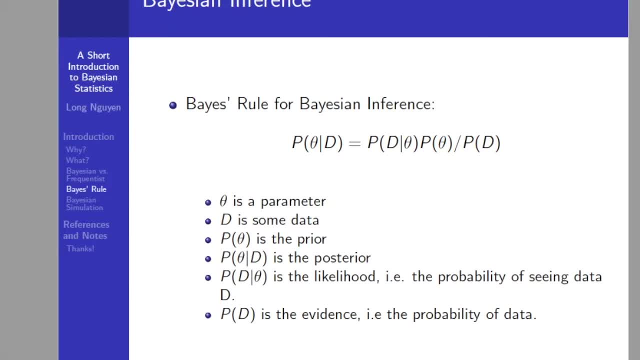 d as generated by a model with parameter theta. For example, if we knew the coin was fair- this tells us the probability seen the number of heads in a particular number of flips. p of d is the added evidence. This is the probability of 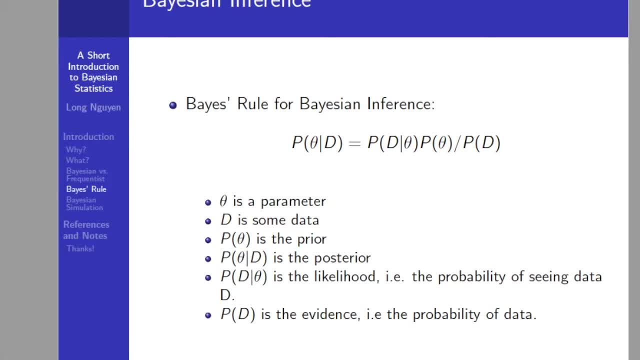 probability of the data as determined by summing or integrating across all possible value of data, weighted by how strongly we believe in those particular values of data. For example, if we had multiple views of what the fairness of the call is but didn't know for sure, then this tells us the probability of seeing a. 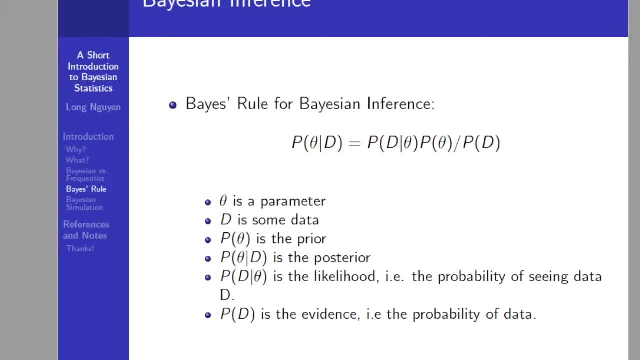 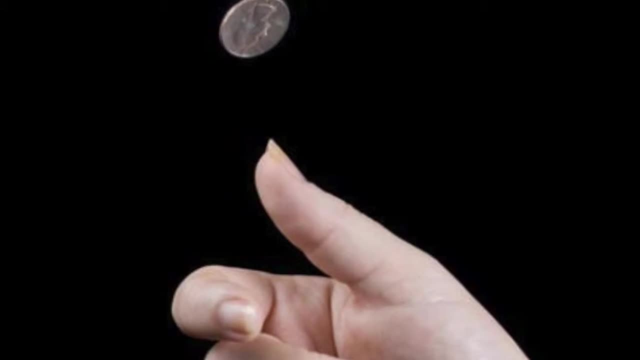 certain sequence of flips, of all possibilities for our belief in the coin fairness. I would like to demonstrate Bayesian inference by a coin flipping example. in this example we are going to consider multiple coin flips of a coin with unknown fairness. We'll use Bayesian inference to update our beliefs on the 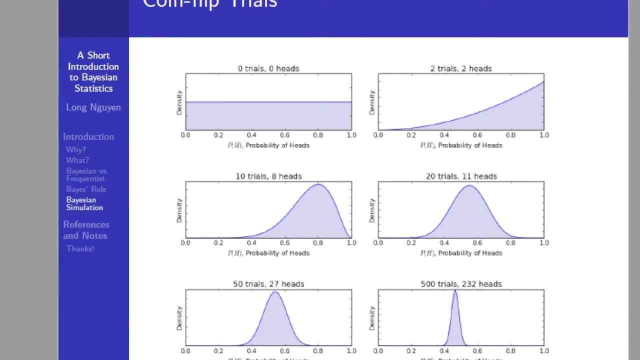 fairness of the coin. as more data or more flips become available, The coin will appear on the other cards and the position vectors can also be seen from the former page. be fair, but we won't learn it until the trials are carried out. Initially, we have 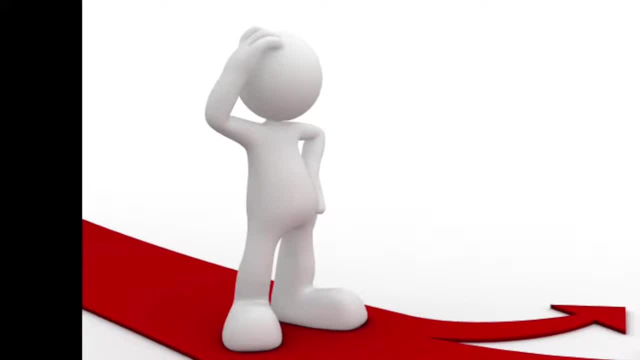 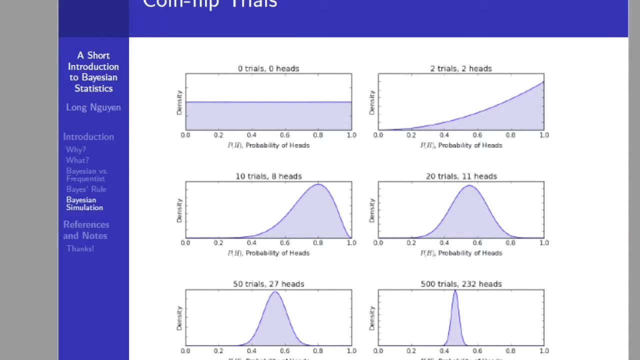 no prior belief on the fairness of the coin, that is, we can say at any level of fairness- is equally likely. We're going to perform n repeated Bernoulli trial with theta equal to 0.5.. We're going to use an uniform distribution as a mean of. 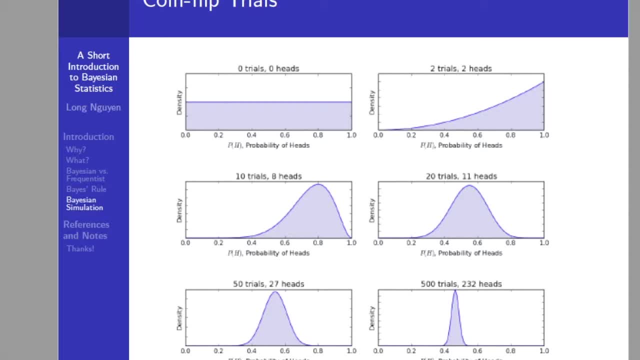 characterizing our prior belief that we are unsure about the fairness. This states that we consider each level of fairness or each value of theta to be equally likely. In the following figure we can see six particular points at which we have carried out a number of Bernoulli trials, or coin flips. In the first graph we 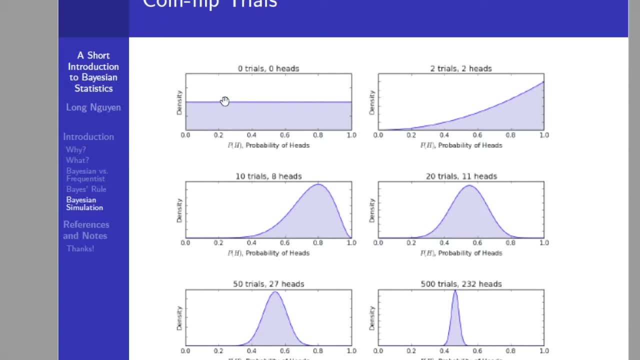 have had no trials enhance our probability density function or prior density. in this case, This is uniform distribution. It states that we have equal beliefs in our values of theta, representing the fairness of the coin. The next chart shows two trials done and they are both heads, As we can see how the weight of the density is now shifted. 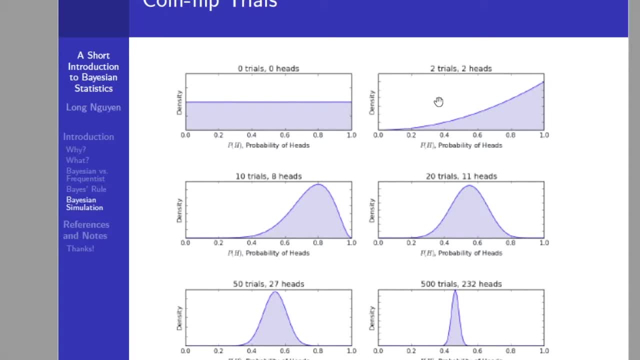 to the right side of the chart. This tells us that our prior belief of equal likelihood counterат col. When we have implemented the�, we believe that the coin is more likely to be unfair and biased toward heads than tails. In the next two charts, ten and twenty trials are done respectively. Although we have seen two tails in ten trials, we still believe that the coin is likely to be unfair and biased towards heads After twenty trials. in the 20 trials, costing hands is common, harder and more likely to lose in these situations and 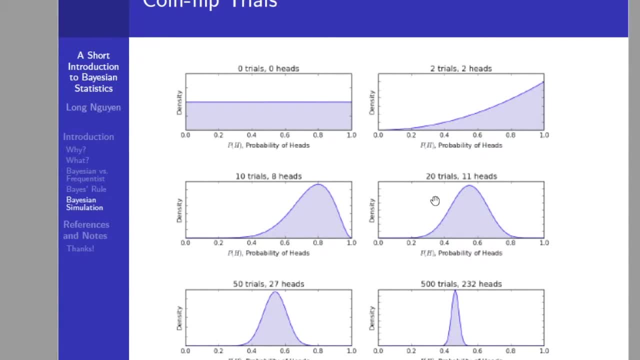 we have seen few more tails. The density of the probability has now shift closer to theta: equal p of h, equal 0.5.. Thus we are now about to believe that it's possible that the coil is fair. After 50 and 500 trials, we now believe that the 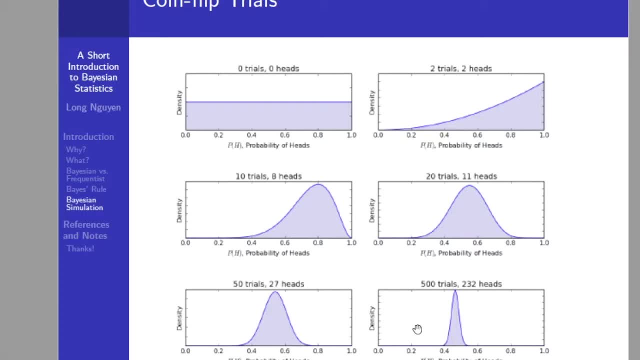 faintness of the coil is very likely, or theta equal 0.5.. The width of the probability density is now staying around theta equal 0.46 in the large chart. If we keep doing more trials, it is very likely that theta approximately 0.5.. Thus, as we can see, Bayesian inference gives us a rational. procedure. So we can see that the probability density of the coil is very likely. If we keep doing more trials, it is very likely that theta equal 0.5.. Thus, as we can see, Bayesian inference gives us a rational procedure. 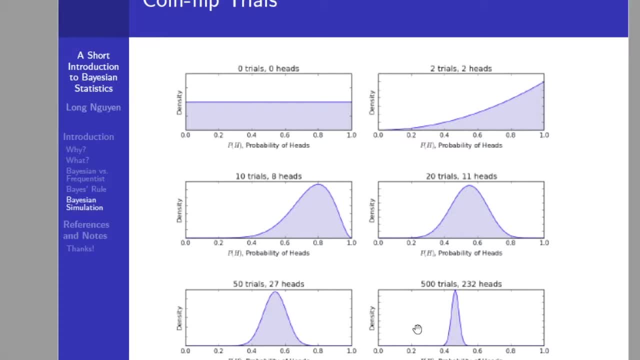 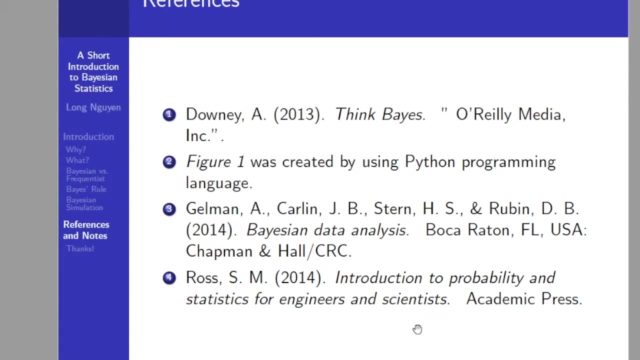 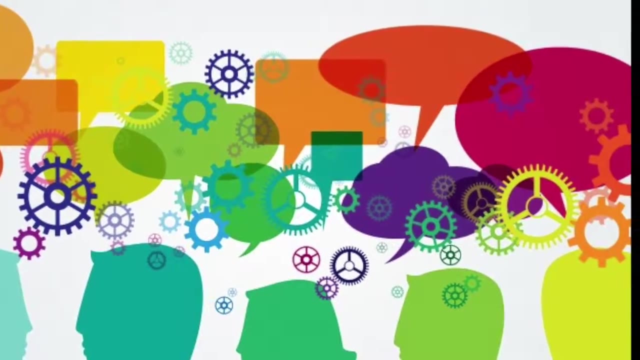 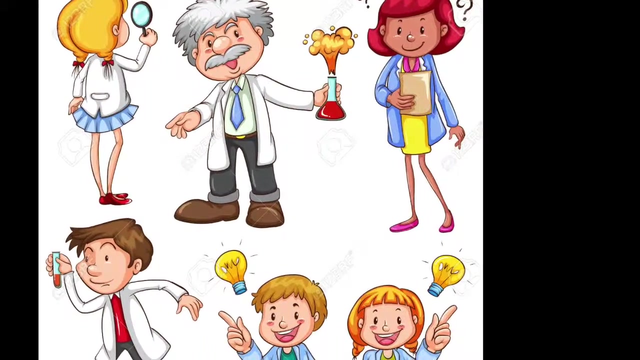 to go from an uncertain situation with limited information to a more certain situation with good amounts of data. In conclusion, in Bayesian statistics, the interpretation of probability is a summary of opinions. A key point is that different persons can have different opinions or different prior beliefs.